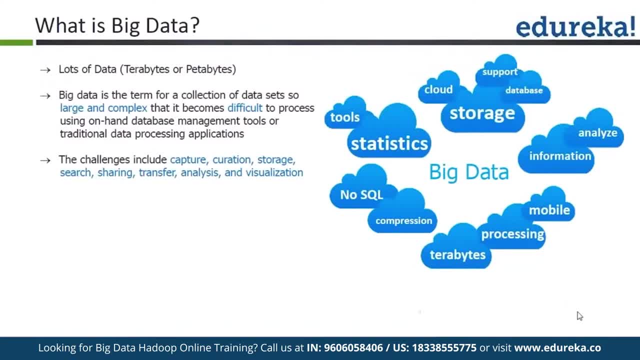 problem. And then you have searching, sharing, transferring, analytics and visualization of the data, All right. So all these, categorically, are termed as big data problem, All right. So time for another story. guys, Another story. If normally, you know, when I go to the webinar, people tell me: OK, I 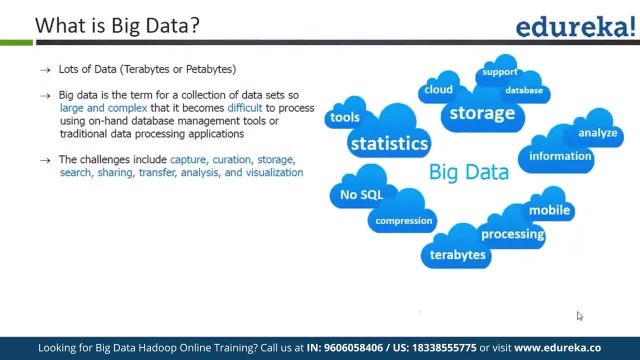 understand what is big data. Now you have been talking about big data and defining big data, But from a layman perspective. give me a use case where big data is important First. all right, Tell me how we can use big data, and things become much more clear when I tell them the story. 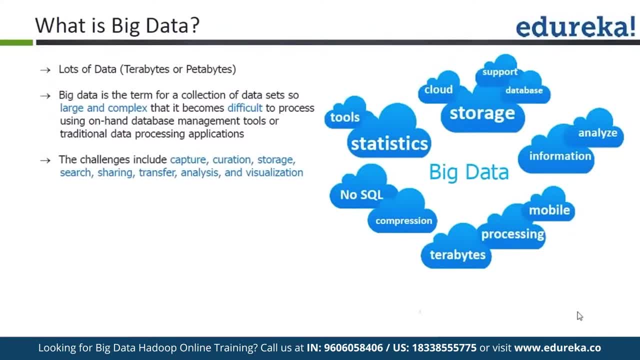 All right, Imagine that all of you are the managers of some bank. All of you are the managers of some bank And, for this quarter, your responsibility is to find out the best possible location where you want to set up an ATM. Now, if imagine that you guys are the managers, what would be your solution? 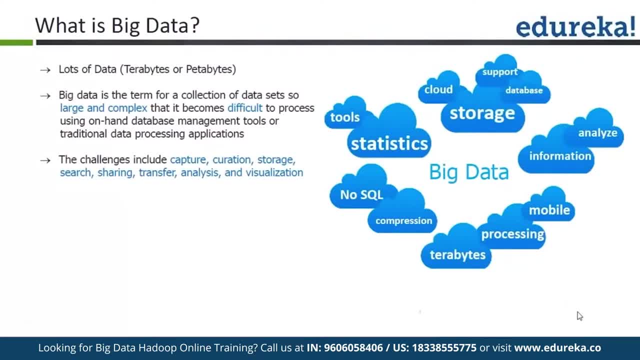 Guys, where do you set up an ATM? What can be your, your solution For that? But if I am a manager, I would say he set up an ATM right in front of my house. You know, every time I go out, every time I come inside my house, I'm going to, you know, go and use an ATM. 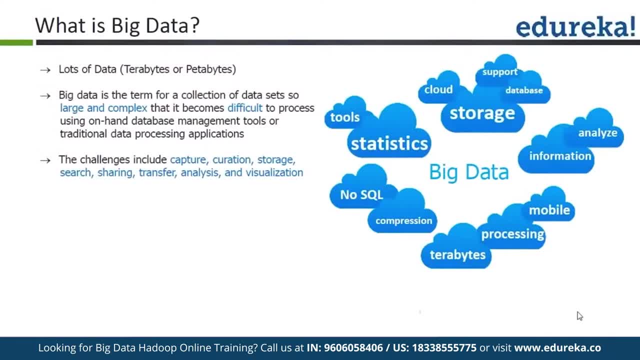 That decision might not be rational. You know it would be for myself as a manager. If I want to become a good manager, if I want to make rational decisions, I just cannot take a decision which is for my own benefit, Right? So I cannot make it. So if I have to become a rational manager, if I have to become a manager who thinks about the company, 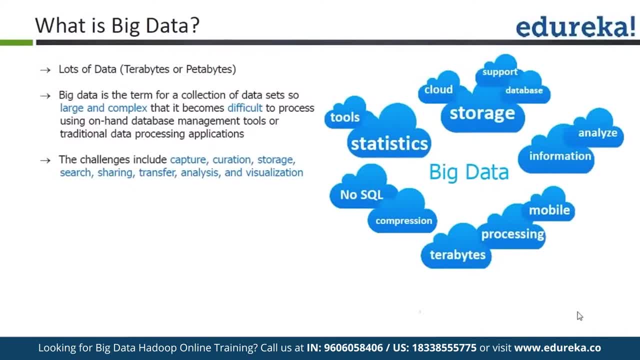 what exactly should I do? What exactly do I need for making a decision? So, guys, what exactly do I need for making a rational decision about putting up an ATM? So you are saying, you know where less ATMs are present, set up an ATM where there is a majority of the population. 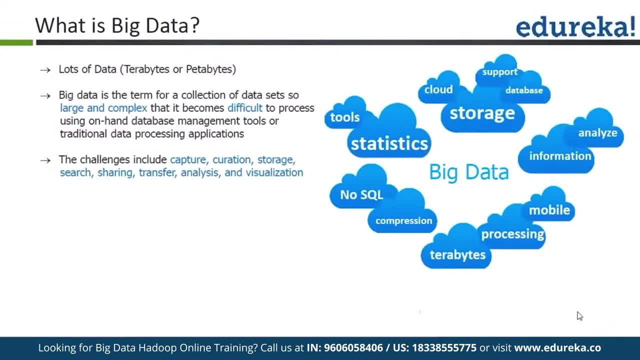 metro station, airport depends on demand. These are the ways of making a decision right. Make it analytics in the requirement. All right, These are ways of making a decision. Perfect. But if I have to make a decision, so let's forget about, let's forget about the bank right now. 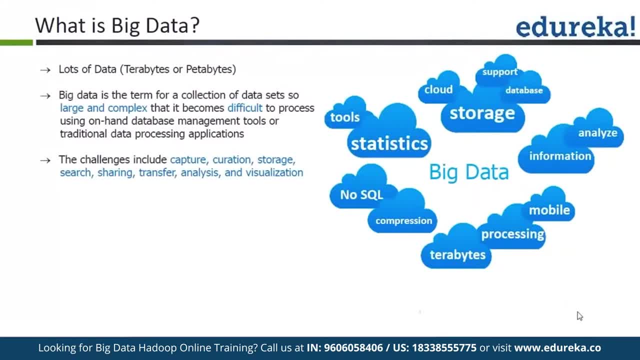 In your life, in your career, in your personal life. if you have to make a decision, guys, what do you rely on for making a decision? What exactly is that important thing that helps you make a decision which is rational? Only thing you need to know for making a decision is the actual data, the related data, 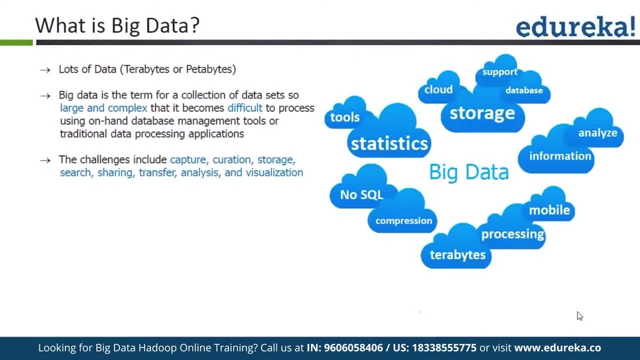 If you know related data, you can make decisions by looking into the data, the data in personal, in personal experience. The data is represented as experience. But these are data also Right, But everything is data. If you have to make a decision, it is nothing but data oriented. 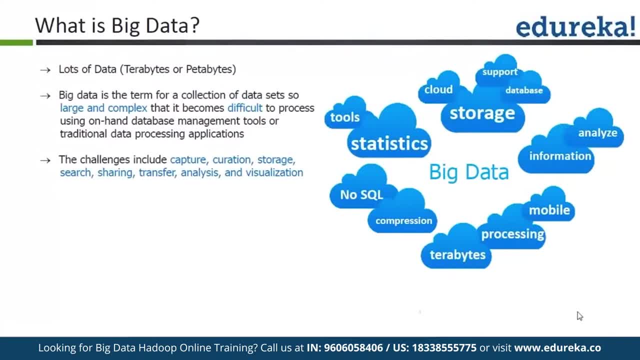 So I, as a manager, I go to my bank tomorrow and I call up my team and I tell them that your responsibility is next week Friday. I want to report where. I want to find out the best locations where I can set up an ATM in the city. 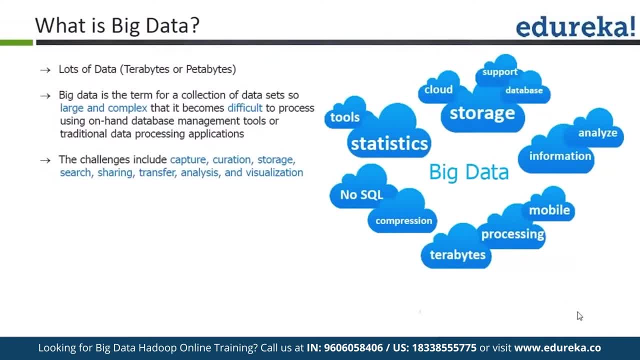 And that's what exactly you want to work on. So I give that responsibility to my analytics team. Analytics team will go ahead and, you know, make a discussion, They'll set up a meeting and imagine that analytics team is based out of our team off. 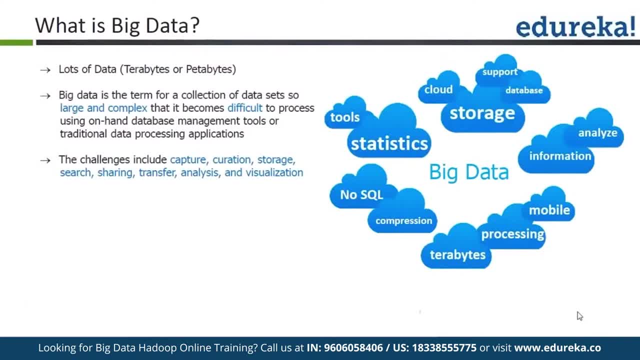 Five, 10 people. they all sit together in a conference room and they start thinking: all right, we need to make a report, We want to make a decision based report, We need data, Perfect. So they agree that they need data. 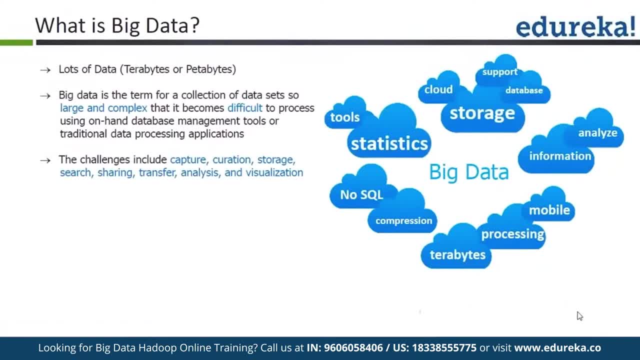 So now the question is: we know that we need data. Where will the data come from? So we have to identify sources of data. All right. The second phase is: and if I want sources of data, can be. So what do you say, guys? 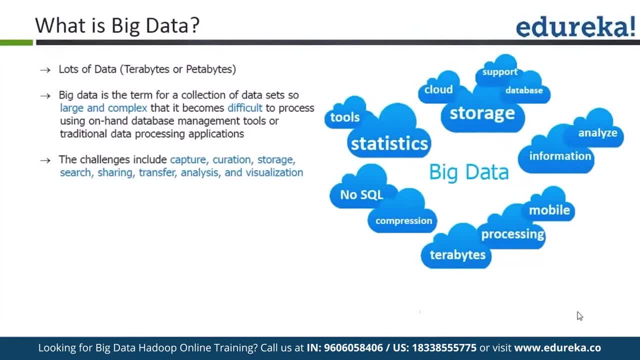 You know what kind of sources of data. I would say the first source of data would be My company's own database. I have my customer customer database. I'm going to pull up my database and find out the data, the customer and their zip code. 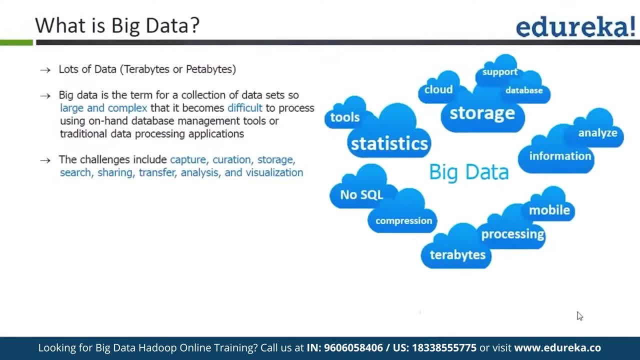 All right, So data internal to my company. So this is perfect. You know I'm getting the data from my company's database, All right. So somebody else and somebody else in the team says: like, what violence has customer complaints? 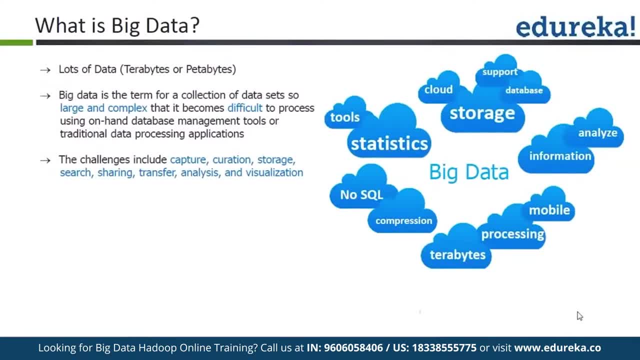 So I'm sure you know a lot of people will be, you know, opening up their net banking or opening up their customer care chat window and chatting with the customer care about and complaining about the lack of medium Right? So yes, I'm going to go ahead and find out logs of customers talking to customer care. 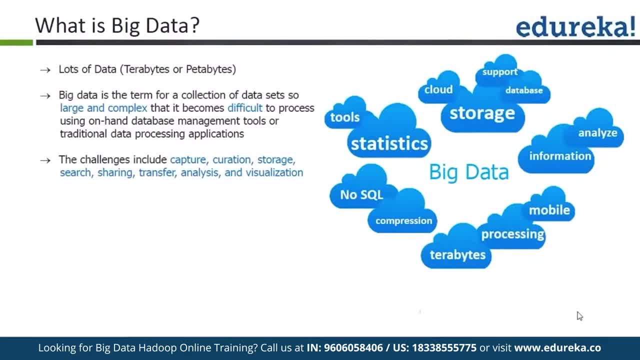 So these logs will be totally free flowing text. Right, This will be unstructured data, totally free flowing text data. You know, normally one to one discussion over over a chat window, These are total unstructured data, But I'm going to fetch all the data from my customer care. 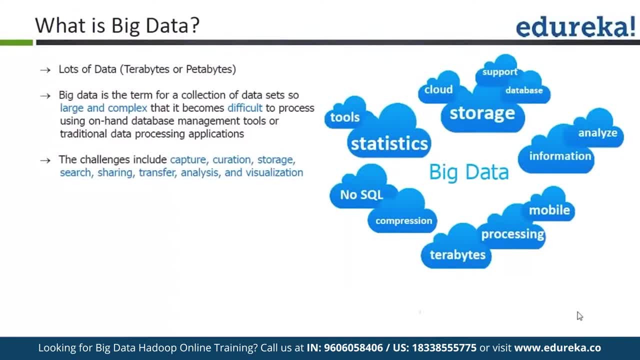 All right, Somebody might have also picked up a phone or the customer care and conveyed the lack of ATM and locality. So second one would be: you know audio files, get out audio files from the customer care. logs for source can be. Oh well, you know, I'm sure somebody might be going into social media and tweeting about lack of medium. 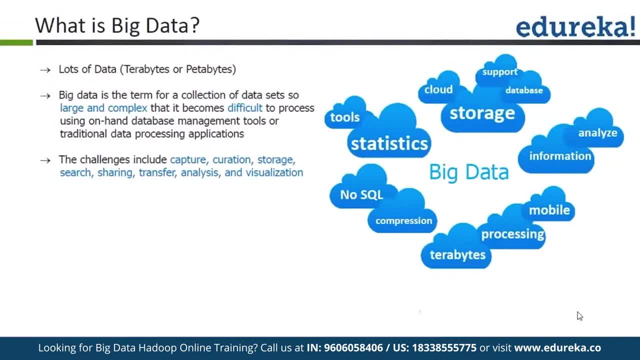 Right, So I can go ahead and search for online tweets or online social media data to find out if somebody is actually, you know, facing problems, unable to look At an ATM. you know survey. So, of course, I can go ahead and distribute pamphlets to everybody who comes to my bank and ask them to fill out a survey. 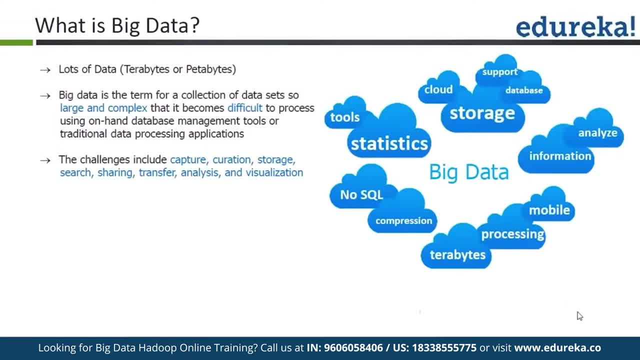 Where do they find a lack of medium in the city, Or I can also have an online survey in my net banking. Every time somebody opens a net banking, I can ask them to fill up a 30 second or a 10 second survey. 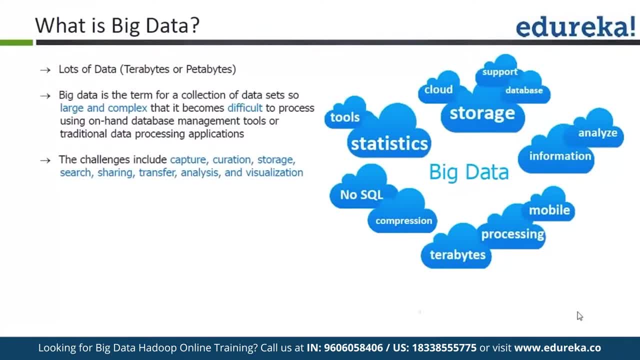 Right. We have multiple sources of data. Data will be coming from multiple sources. if I want to make a rational decision, I cannot I rely on my, on my, on making a decision only on one source of data. that will not be rational decision. 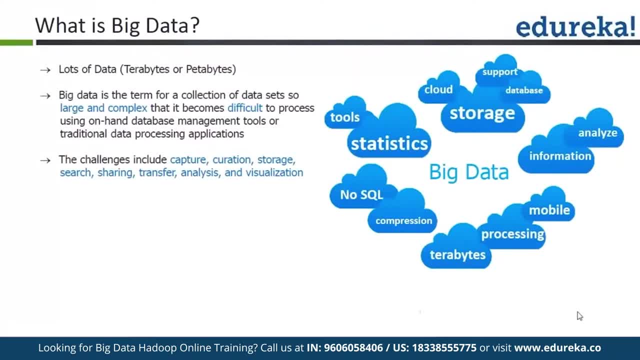 If I want to make a rational decision, if I want to really make a correct decision, I have to look into the data that's coming from all those sources and collectively make a decision by looking into this data on a whole Right, A 360 degree view of the data. 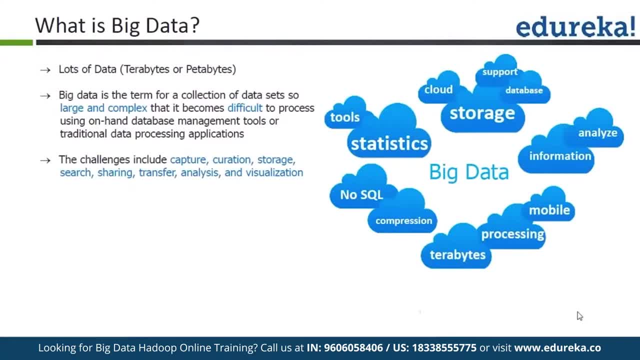 I have to collect data from all the sources and then make a decision. So my question is now: this is where we have defined the problem. Question is: somebody will say, hey, where can? What can be a solution, What can be a solution which can allow us to do that? 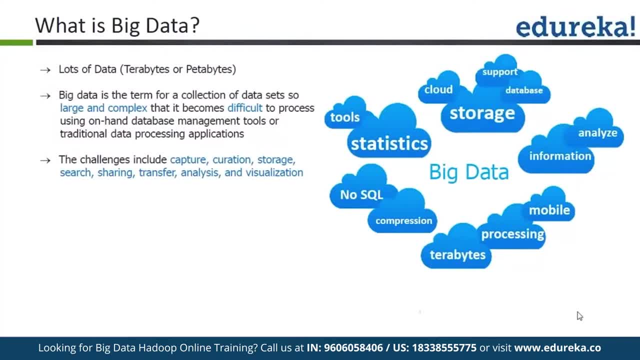 And can a database load data from all those sources? It cannot. It cannot store Right, It cannot store data coming from all those sources and have a unified view. Cannot have it, You cannot have it. So we all agree that this analytics team are limited by the progress of the software technology. 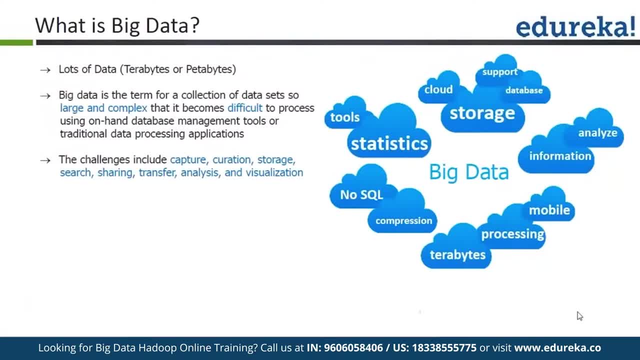 They are limited by traditional systems. Right, Traditional systems will not allow them to collect data from all the different sources And look into the data holistically. It is impossible. So maybe out of 10, somebody says: hey, I have heard about something called Hadoop. 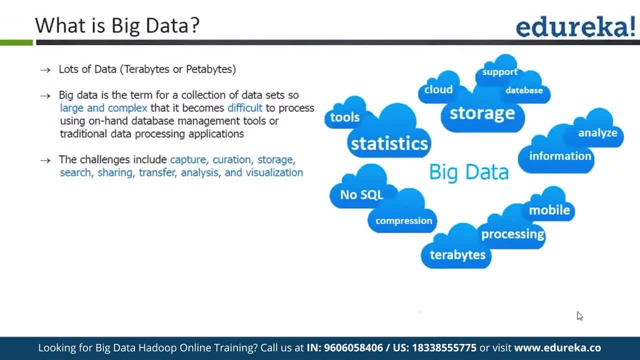 Hadoop is a new technology. Hadoop is a solution that does give two things. Hadoop is a solution that gives two things at the bare minimum. One is it is a platform where you can load any kind of data And secondly, it allows you to write processing algorithms on that large amount of data. 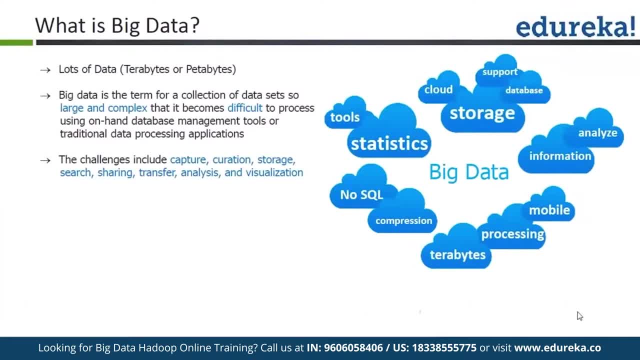 So Hadoop is a platform that allows you to store all of all the data that you think about And it gives you a platform for processing the data that you have stored. So these guys in the analytics team in that room they thought, OK, this is a correct. 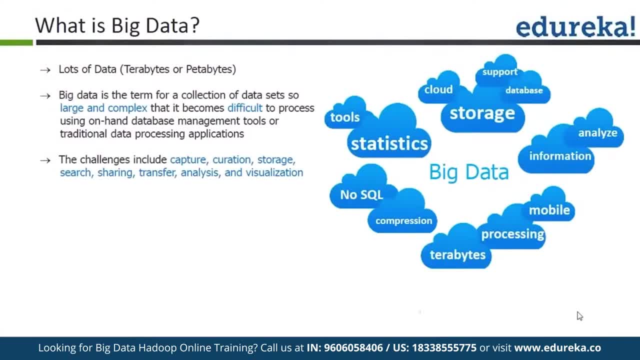 use case for big data. So we have identified that, yes, if you really need to have a platform, a solution where you can collect data from all the sources and process it, then there is no other technology apart from Hadoop that can do it right now. 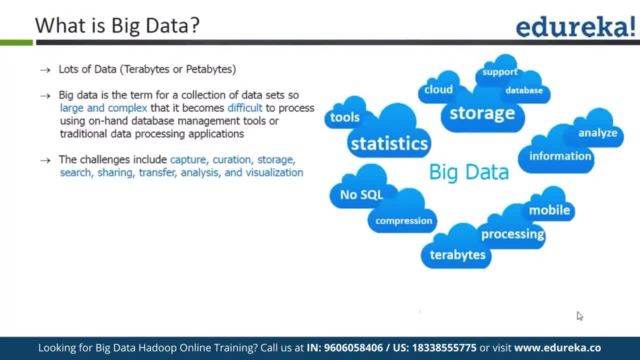 All right. So what this team do is they collect data from different sources, store the data into Hadoop And then they create a report in Hadoop And the report will have maybe a chart saying that the most important area or the top of 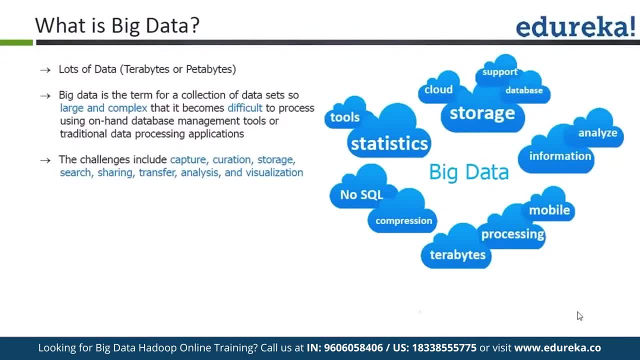 the list area where you need to set up an ATM will be ABC location And the second in line would be XYZ location. You take the report, you come to the manager. The manager looks into this report and says, hey, I have got what I need. 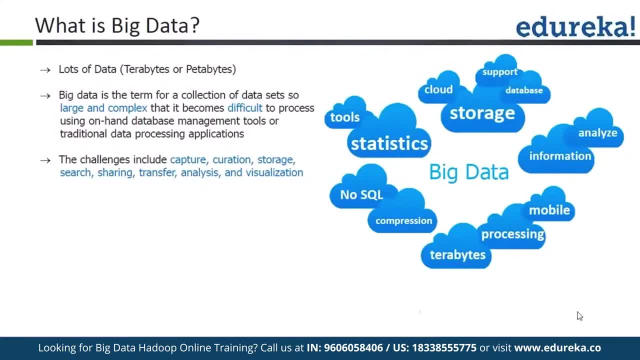 Now what I do is I can go ahead and make a rational decision. My decision would be: set up an ATM in ABC location Each quarter. if I really want to set up another ATM, I would go and say, hey, go and set up an ATM in XYZ location. 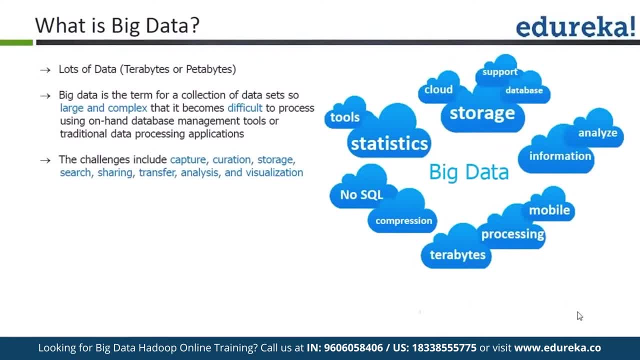 All right, So this is how big data Hadoop solves actual business problem. So what does big data Hadoop tries to do? Big data Hadoop tries to provide a decision making capability by loading and storing large amount of data. All right, So it is a data processing platform that allows you to process large amount of data, irrespective. 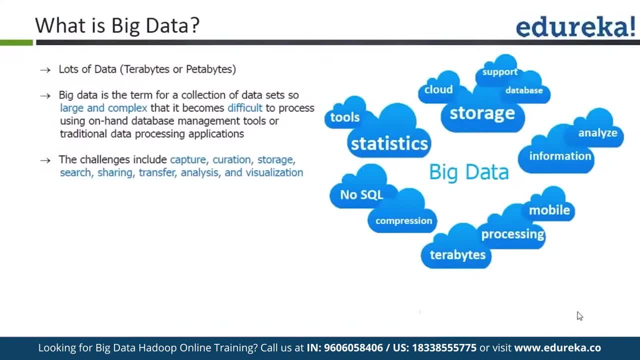 of how much of data you have in a very fast and timely manner. So this is how big data Hadoop tries to do. All right, So what Hadoop does is it tries to do a decision making in a very timely manner- because you are even not worried about the processing capabilities right now- and try to provide 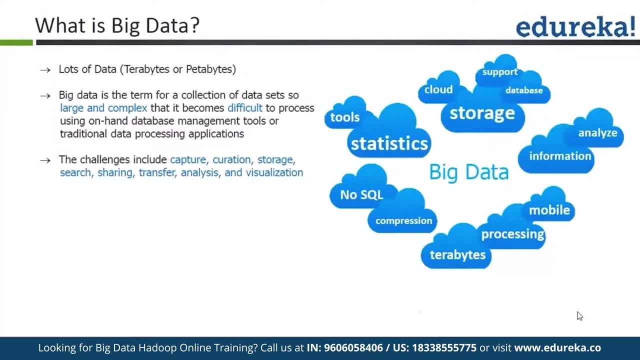 a solution which is used for business decision making. So Hadoop is an analytical software guys. It is not a point of sale software, It is not a web software, It is not a customer oriented software in that way. It is an out and out analytics software. 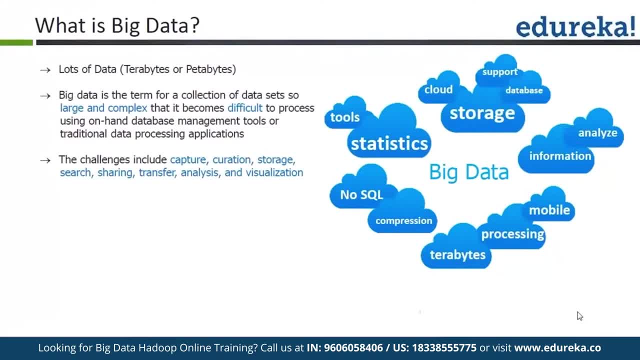 It is used for making or deriving hidden patterns in the data so that the management, the business, can make decisions of the business, the business grow by looking into these store data. all right, so it is an analytic software used only to ensure that it can help make a decision on the 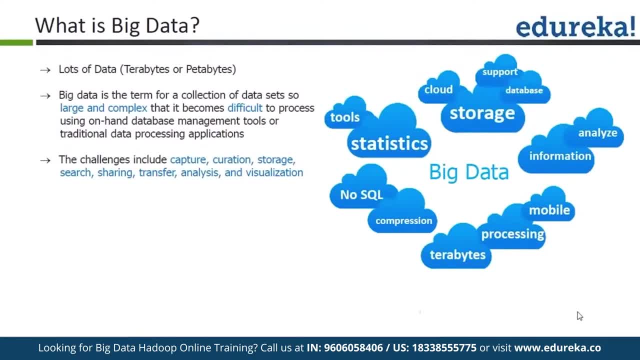 business front right. so it is a business driven analytic software- how data like video images used to store in Oracle before Hadoop. well, honestly, guys, honestly, nobody is to save images and videos in Oracle. what they used to do is normally they'll store the images in the videos in a cloud based system and store. 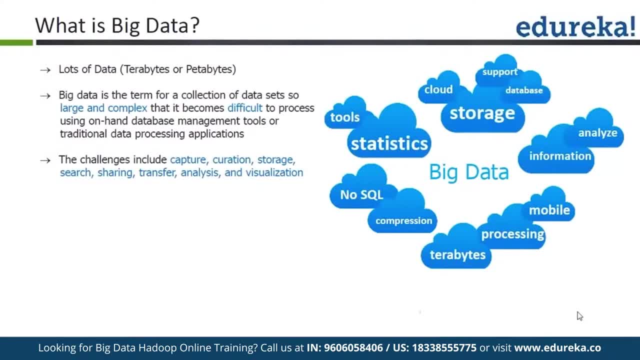 the URL in one of the columns in, you know, in your database. so database normally do not store images. you know it's a very bad design. normally people do not do that. they have an image server. they have us some kind of a public based, you know cloud solutions where they'll upload the videos and everything. 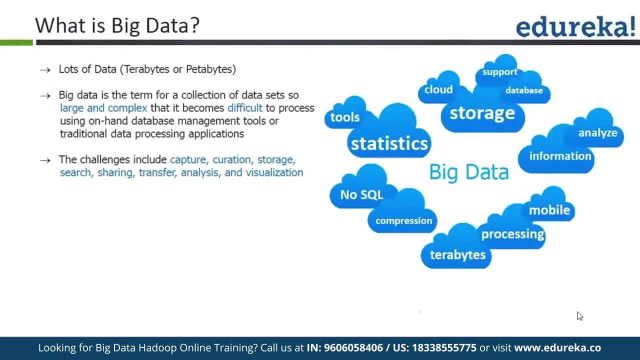 they want and only the URL will be stored into this RDBMS. you know I've seen people you know saving smaller images as blob objects. you know you can save images as blob objects and you can save images as, but tremendously slow. that's a very known strict no-no into you know data. 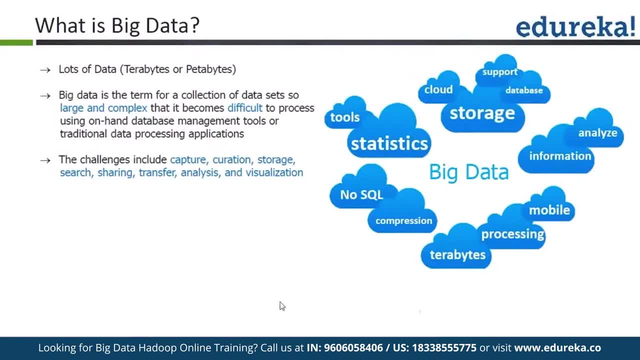 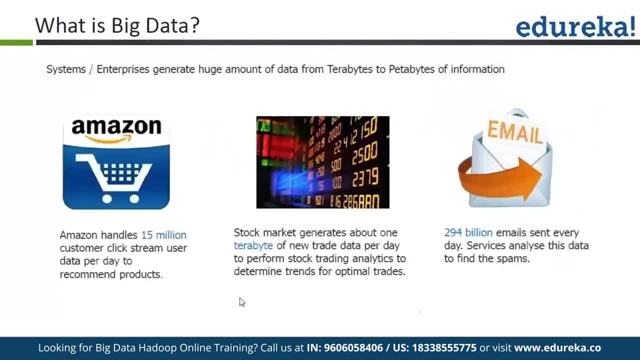 modeling right, so nobody does it. Viadam says: can you analyze audio-visual files using Hadoop? the answer is yes. so what is big data? we all have unidentified. so you know, Amazon handles 15 billion customer clicks per system, you know, or on a per day. so basically, if you go into any other, is it possible to? 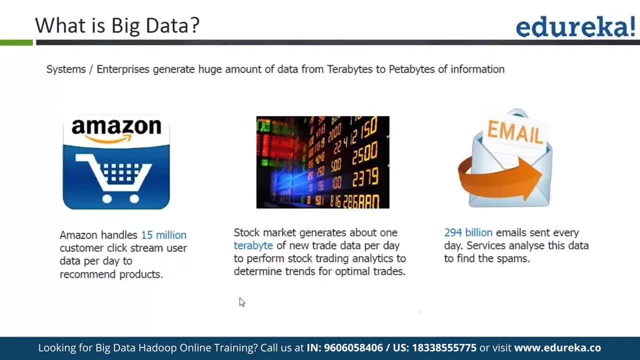 view others question. yeah, unfortunately you cannot view others question and that is the reason. you know, every time somebody asked me a question, I repeat the question, I read it out loud, all right, but I unfortunately we cannot. all right, yeah, so what is big data? so we have been seeing big data in 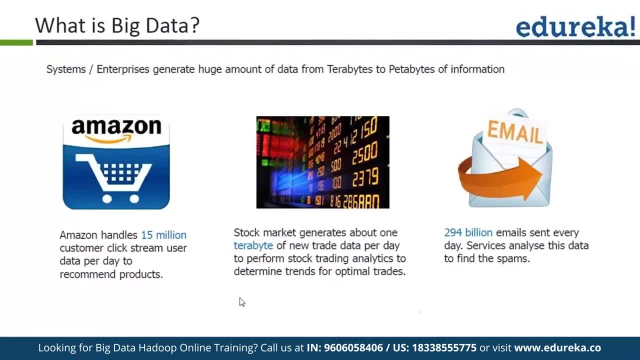 a lot of different places and if you go to Amazon and you go to Best Buy, you go to any other. you know retail websites, all using big data. stock market- well, New York Stock Exchange, ncdc, you know they're using the non-stop, they're using big data for analytics of stock trends. and then two hundred and ninety four. 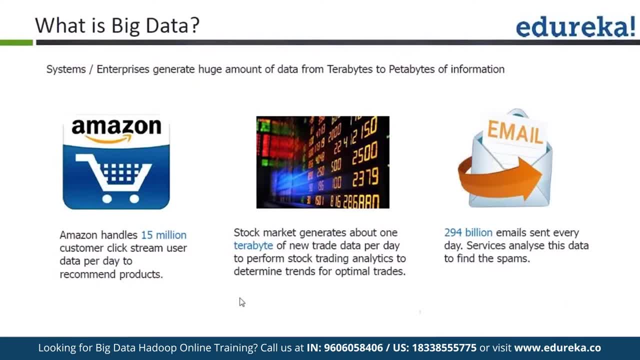 billion emails sent over every day. so huge amount of email sent. and how do you filter out the data? so, while the use case is, imagine that you have a very large company in your company, of course, will be receiving a large amount of emails, you have to, you know, find out whether the email is a spam or not, right? 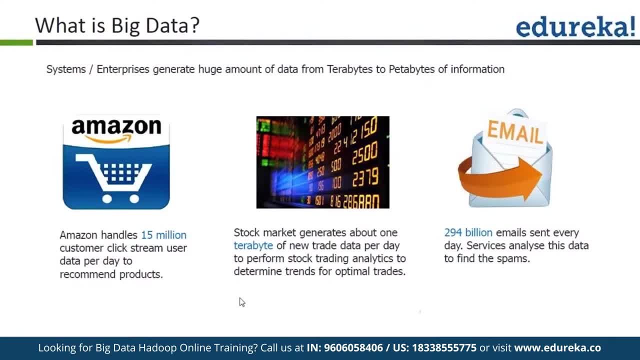 so your mail server have to make a decision whether the email is spam email or not a spam email. so what do you do? right, you cannot open the email. you know in a traditional system, and this you know: read the email and see whether spam or not. so you have to do, you have to. 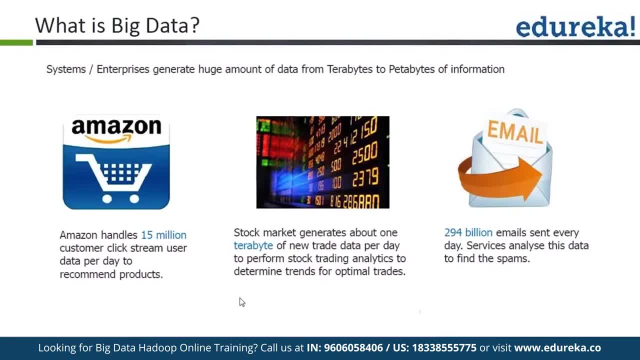 provide a system which is a distributed system with large amount of processing capabilities, so that on a real time, you can find out whether the email is spam or not, right? so all in our use case of big data. we're going to talk about the other use cases of big data as we move along, but, all in all, what I'm trying to 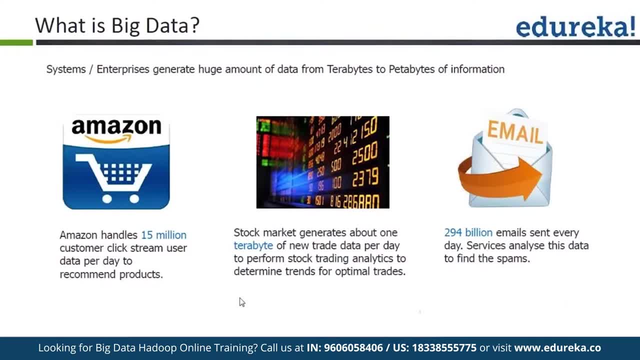 say, is: big data is available in your surroundings. you know, when you look up in your, in our surroundings, everything you do, everything you work with in today's world, has a big data angle to it already right so, even though of a, we think about big data as pretty new, but it has been there for quite some time. 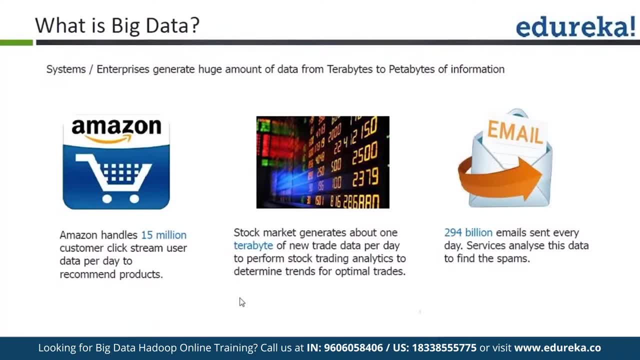 and people have been using big data for almost lot of time right now and a lot of systems have been developed and- and I have gone live into production with big data's. big data is very stable. it is doing wonders. all the companies, all of the top hundred companies, have already migrated to the data. they are using big 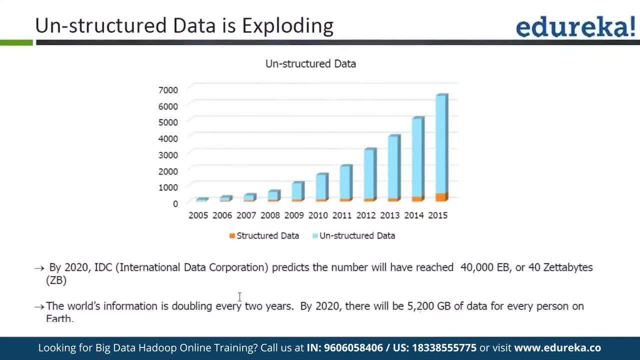 data and they're using it for true. so one thing about big data is: it is not a technology. big data is a problem statement, the platform: nowhere we have mentioned that it is a software bundle. nowhere we have mentioned that it is a tool. so, to be to be very honest, guys, i started my career in big data five years back. 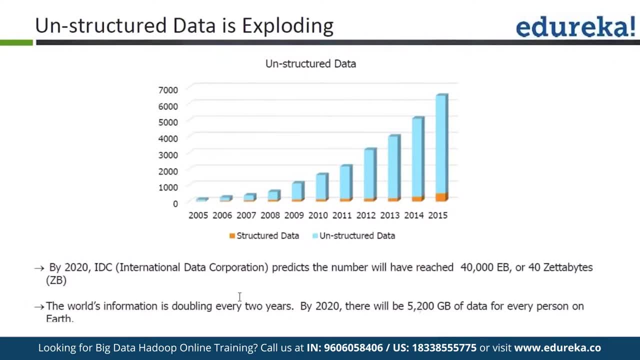 and if i tell you about the things that i have learned in the last you know, or i've learned on the first year that i've joined big data, you guys even do not know about the names because they have been obsolete by now. so in big data environment, guys, you have to keep your mind open that every 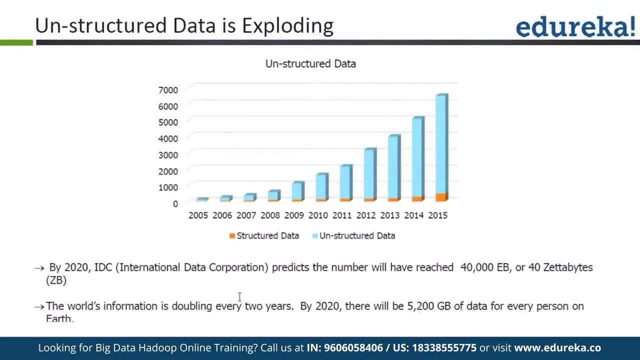 three months you're going to think about, you're going to learn about and you have to upskill yourself into new technologies. so big data is not a technology, it is a platform. in that platform, you're going to have new technologies coming up: the internal architecture, the basic architecture. 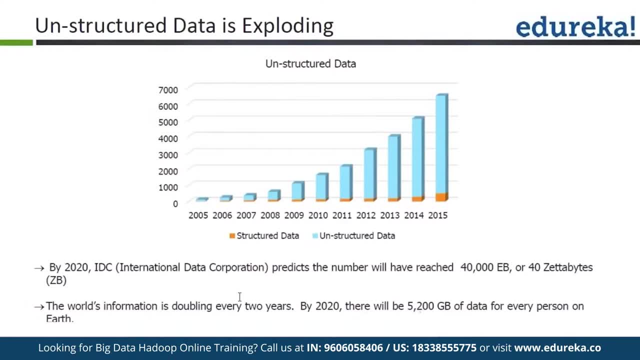 is going to remain the same. we're coming up. as you know, you cannot even imagine the rate in which things become old and new things pop up right. so in big data world, you cannot just, you know, hold on to the past law and say, hey, i've learned about it and i'm going to be pretty okay with it. 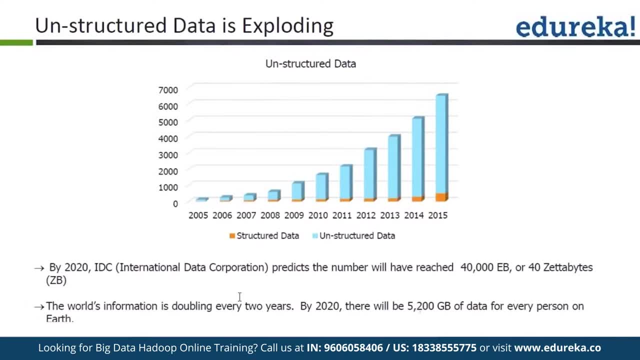 for next five years. no, in big data world, the concepts are important. when you learn the concepts, the services, the softwares, they're going to change every three months. that's how it is, you know, for the last five years. every three months there's something that new comes up, and then data, if you 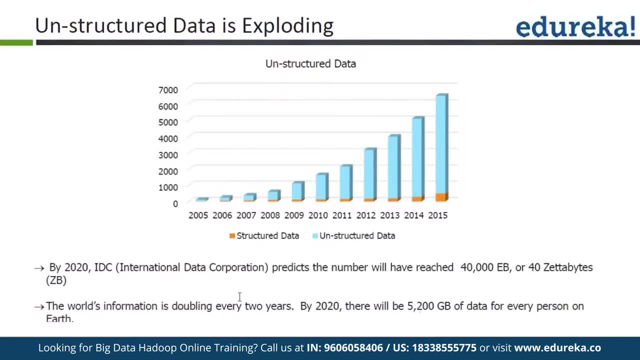 want to be in the technology world. if you really really think about understanding the back end of the data system, then big data is for you, because big data, you know, is not reliable to a particular software. there is not a single software that is associated with big data, whereas 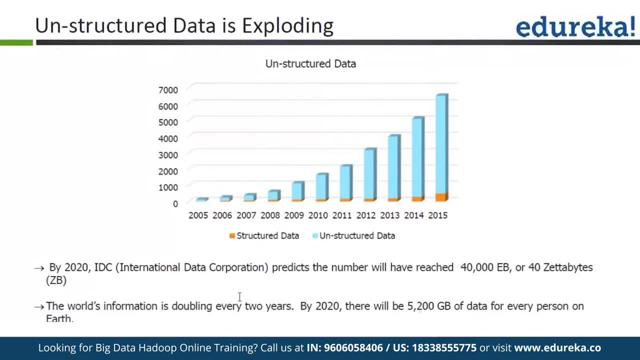 it is just a platform and that platform gives you advantage of learning new things. you know, if you are basic secular, you can learn. and you know, get over with the news use case: a new service very soon. so what exactly is big data? so let's look at this graph, guys. in this graph, it talks about the trend. 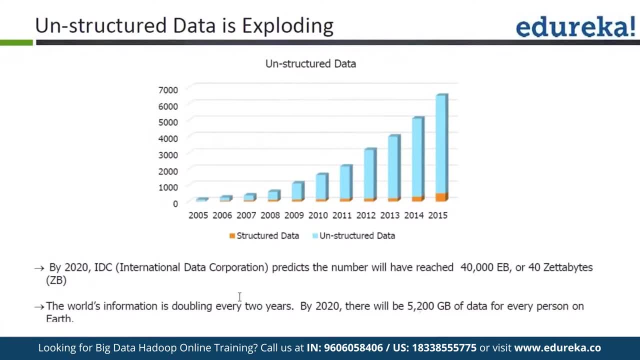 of data. all right. so starting from 2005, people have been seeing a large amount of growth in data. now if you classify the data, you can classify the data into two different segments. one is structured data. what is structured data? structured: the data which is already available in your system. you know. 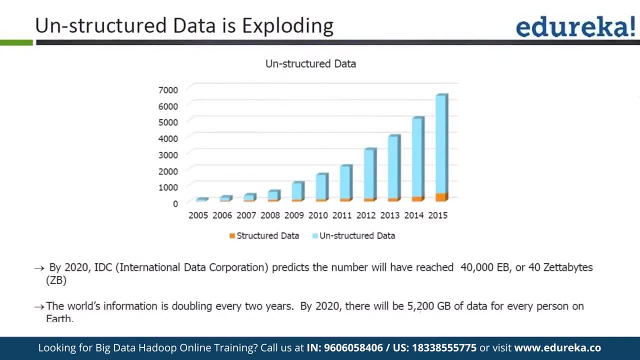 your relational data system, all your rdbms back system. these are all storing your structured data. if you look into the structured data, you'll find that there is a linear growth of the structured data for last 10 years. last 10 years there has been a linear growth of the structured data. if 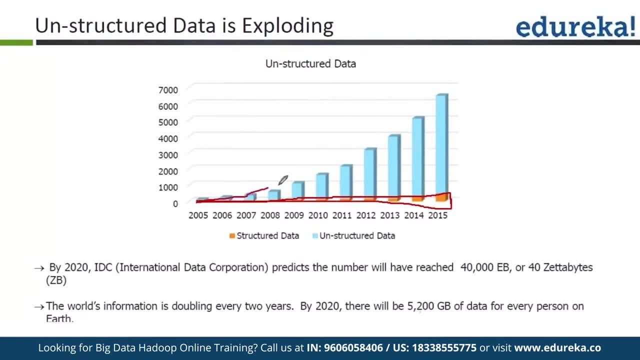 you look into the other phase of the data, have seen that data has been growing exponentially for last 10 years into this unstructured data. unstructured data are all the data which are outside the scope of your system but freely available, like social media data, email data. you know all your. you know internet based data every. 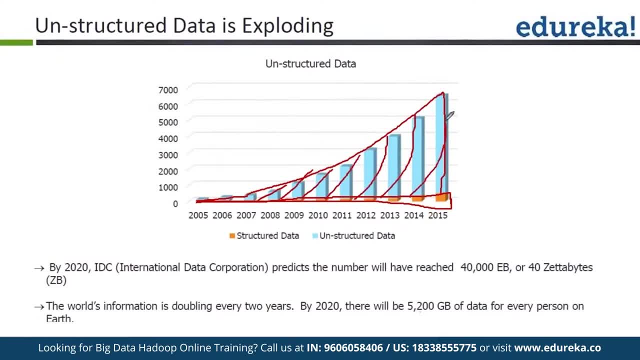 single data which is outside the scope of your organization are termed as unstructured data and people have seen that there is a exponential growth of the data. what has happened in 2005 that you can see that there is an exponential growth in in this unstructured data? that has happened in 2005. 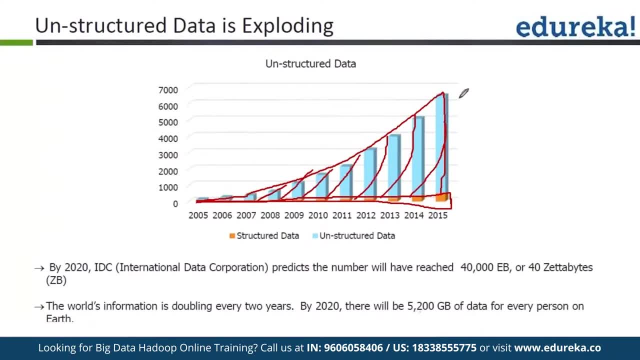 facebook went live. social media: yes, the same thing. right. so 2005 was where people went to web 2.0, where people are talking about, in all the social medias, all the mobile applications- everything was, you know, coming up. so it was a huge boom in the data management systems, right? so, starting from, 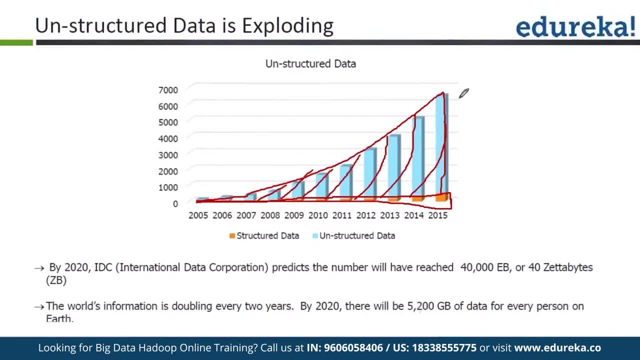 2005, you see an exponential growth in the data. imagine that you are supposed to make a decision in the business. you know your business is supposed to make a decision. can you rely only on the 10 percent of the data, guys? do you think you can rely only on the 10 percent of the data to make a decision? will that decision? 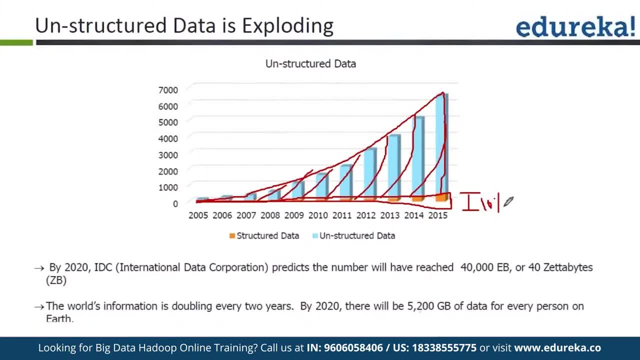 be correct. probably, yes, probably. the decision will be 10 correct. if you're only looking into 10 percent of the data, 90 percent of the time your decisions are going to be wrong. similarly, you cannot also rely on only the 90 percent of the data so to make a decision in today's world. 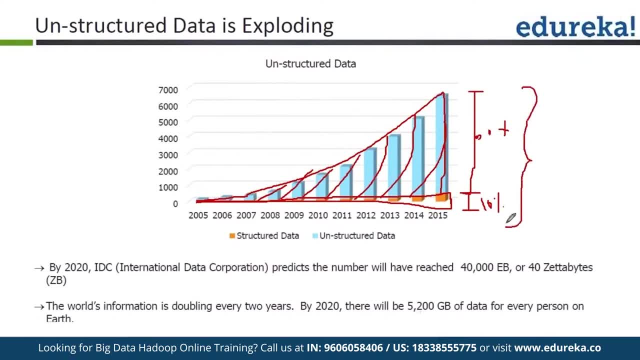 you have to rely on all the 100 percent of the data, so you need to find out a platform that can process structured data as well as unstructured data, that can combine structured data as well as unstructured data, if there is a platform that can look up, load all these kinds of data together. 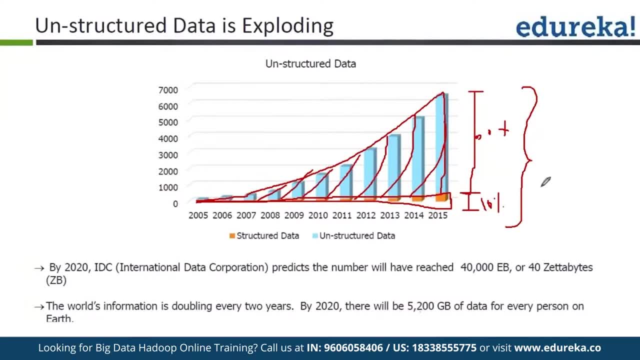 then that decision making system, that system will definitely help you make any kind of decision that you think about, because decisions are backed out only by the data. so data collection, processing and analytics can be made, you know sure, only when you collect all different kinds of data and process together holistically, right? so this is the analogy why. 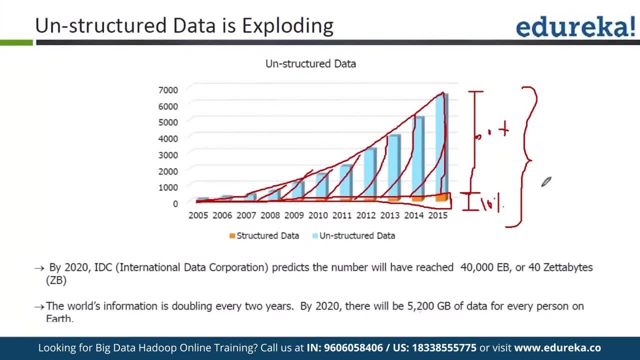 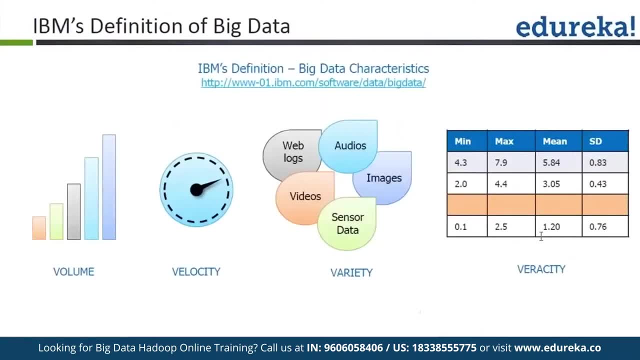 you need to do with data, one trend of data. it cannot just rely on the structured data or only on unstructured data. you have to combine both these views together and see a holistic view of data. uh viram says: does company give more preference to analytics from structured data? 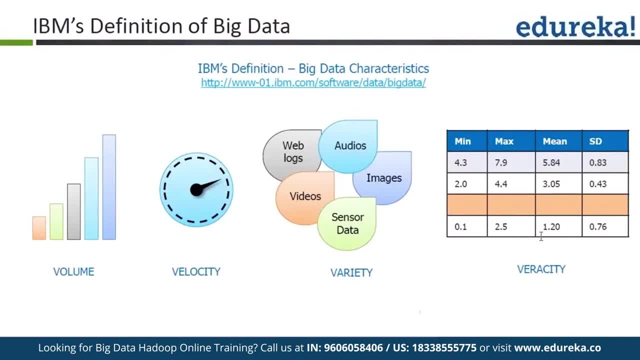 than unstructured data. yes and no, yes and no. all right. so why yes and no? again, we know the percentage, the data that is stored into your structured traditional system in your company. these are only 10 percent of the data, right? these are only 10 percent of the data. 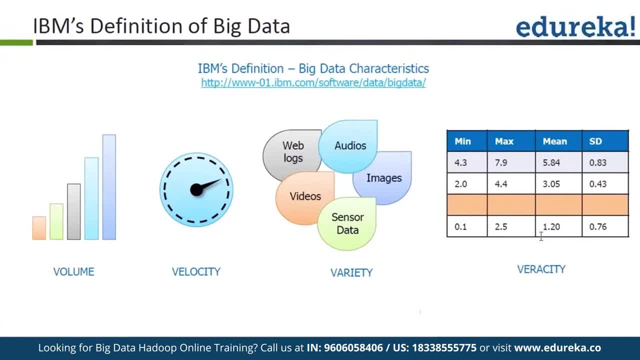 but, most importantly, these 10 percent of the data are all genuine data, very important data, where the other part of the story is 90 percent of unstructured social media data. so, although the number is 90 percent, relative data from that 90 percent. when you have to, you know, crunch down the. 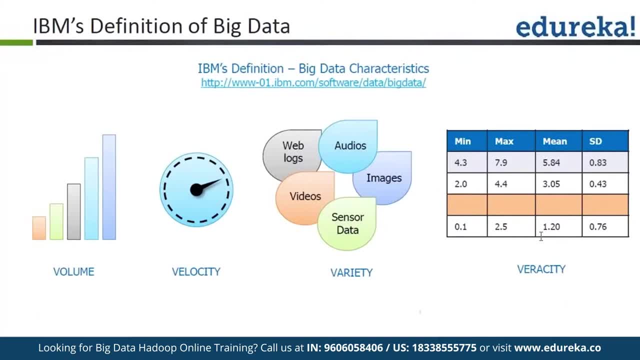 numbers. when you have to analyze the 90 percent, you will see that it is only 20, 25 percent of this 90 percent. that makes sense to you, right? so, all in all, a company has to give equal weightage, but unstructured data will have to be, you know, analyzed more because you do not know what value. 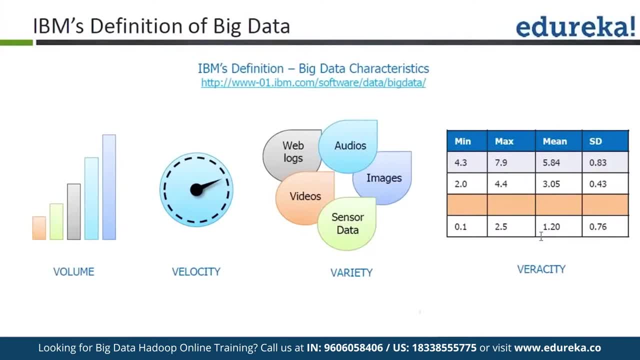 that data stores right, unstructured data, social media data- will not have large amount of value. it will have limited amount. compared to 90 percent, the data value would be very less, whereas the 10 percent of the data- these are all actual, real, really important data. so, whole in all, 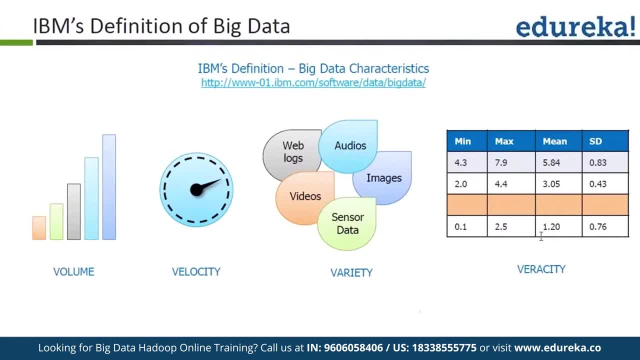 you know, you cannot rely on only one page, and if you think 90 is good enough, i can ignore my internal data. well, no, you cannot do that. similarly, you cannot just ignore social media data. i'll tell you a story, guys again. another story now. imagine that you know. 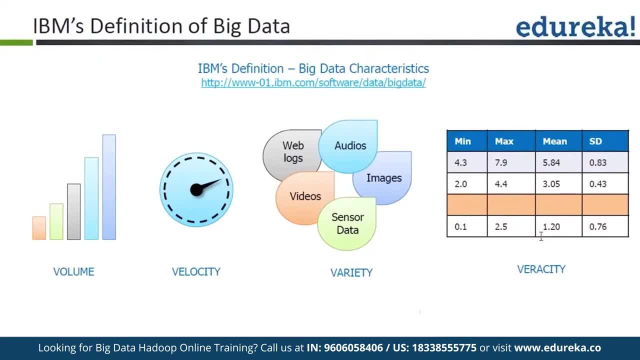 imagine, in a virus you you go to a local shop that you have been going for last 10 years, right? so vyron goes to a local shop that he has been visiting last 10 years and he wants to buy a bar of chocolate, and he really wants to buy a bike in a bar of chocolate. he goes to the shop and he 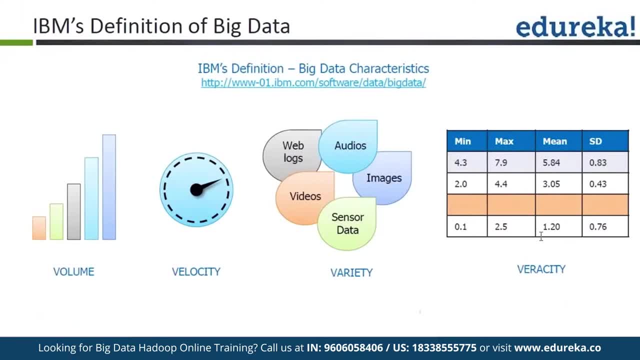 searches for a place where he goes and buys that you know, picks up that, a bar of chocolate. so every time he uses the system has an intrinsic and an extrinsic need. what are the extrinsic needs of viron? what can be the extrinsic need? simple, right. the extrinsic need is the chocolate. yeah, the bar. 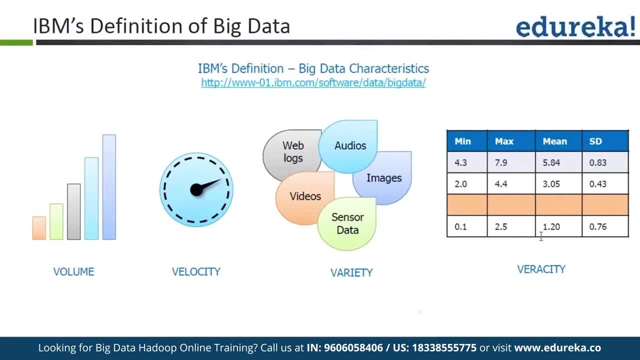 of chocolate is the extrinsic need. he has gone in for buying that only. what is the intrinsic need of viron intrinsic need would be because he's been going to that shop for last 10 years. he thinks that the store owner will at least say: hey, mr, you know, uh, viron, how are you doing today? you know a? 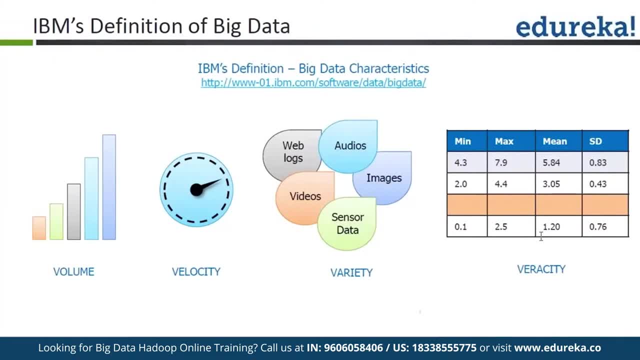 relationship. or he can say: hey, viron, you know, i have this store counter open, even though there are a couple of like people in the line. he says: vitamin, can you come here, i can quickly build you up. intrinsic need is he wants to get a personalized touch from that store because he has been frequent. 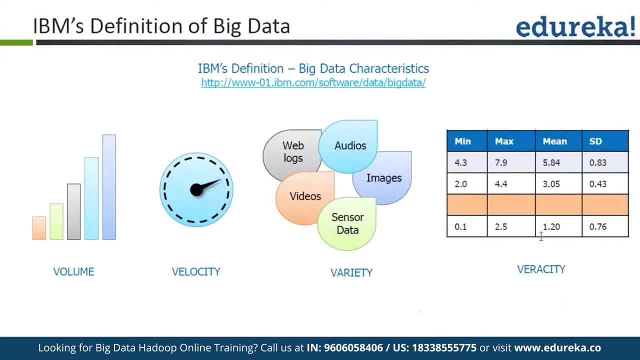 frequenting the store so much. if i've been going to the same shop again and again, i expect that the shop owner gives me a little bit more than anybody else. that is the difference. in today's world, you just keep your customers, you know, happy only by fulfilling their extrinsic needs. you have to. 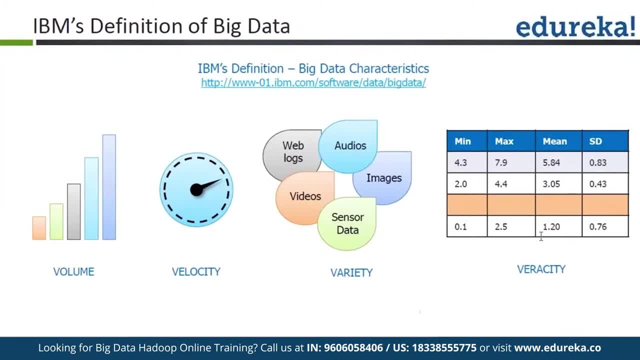 cater to their intrinsic needs. you have to understand what they want before they come and tell you that's what apple has been doing right. so apple has in going and becoming such a huge industry right now company because they give something to you before you go and demand it. 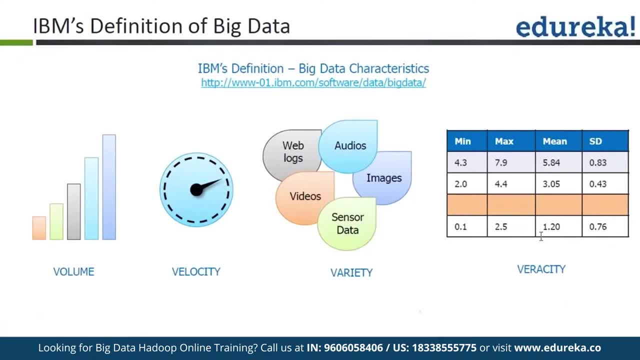 you know that is the reason they have such a good and such a loyal customer following or customer base, because you're thinking about the customer first, right now, right, so your so in order to find out that intrinsic need. in today's world, when people are talking about online based- you know shopping and all intrinsic needs can be found out. 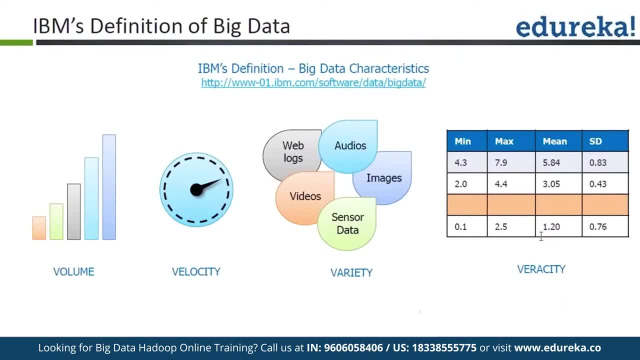 only by looking into your social media and other data, data which is outside the scope of your system, outside your relational world. your relational database will have extensive needs- who has bought what? but your intrinsic needs can be only found out from outside the organization, which is, of course, from social media and all other things. 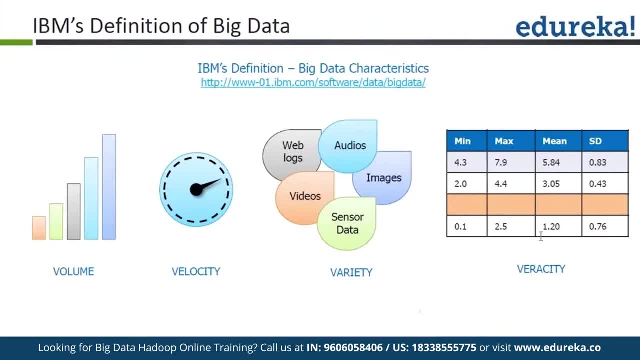 right, and that is why you have to combine your extrinsic need data, which is social media data, along with extrinsic data, which is a relational data, and combine those two and find out the dynamics so that you can cater to the customers better. so no data is important. no data is. 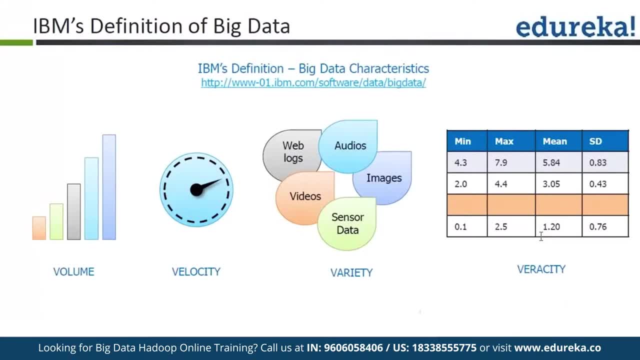 unimportant. everybody has to cater to customer need and it has. it will come from both these sides of the story. it has to come from relational world and it has to come from a non-relational world also. all right, now, you guys? no big data. You have heard about stories of big data. I know you have been now thinking. 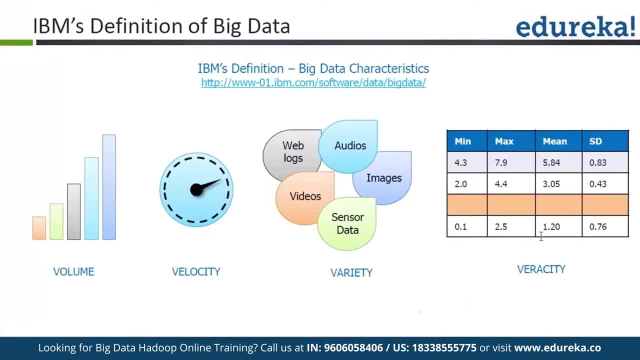 a lot about big data. We imagine that all of us are here to become tech arcs in Hadoop, right? So we want to become technology architects in Hadoop. Imagine that we all are technology architects in Hadoop. We go to a client place and the client says: I have a business problem. 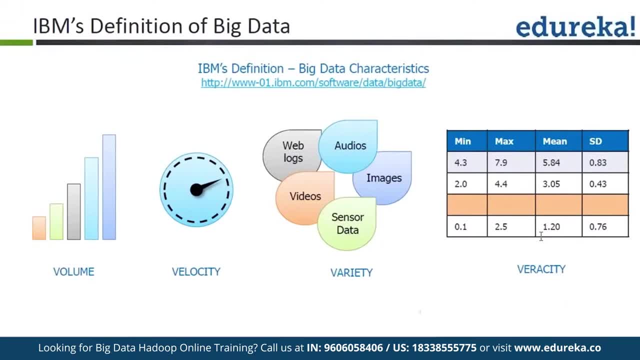 So what do you say? Do you say, hey, I know Hadoop, I do not need to know your business problem, Go with Hadoop. I can tell a customer that they need Hadoop, no matter what problems they do have. Probably not right. You have to find out whether Hadoop is the best suitable. 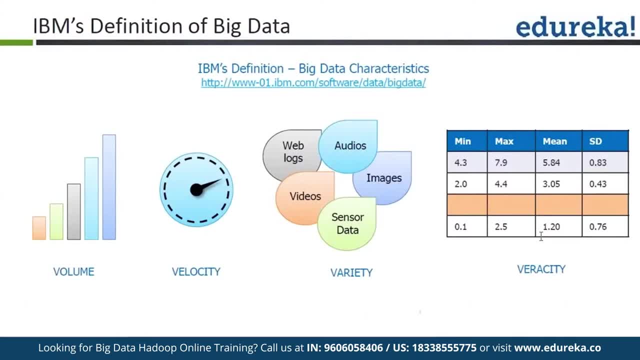 fit for their business, problem or not. You cannot just go and propose Hadoop to everybody. It is not the way right. You have learned Hadoop Now. this is the latest technology you are learning. If anybody says, hey, I have a problem, you say, hey, Hadoop is the. 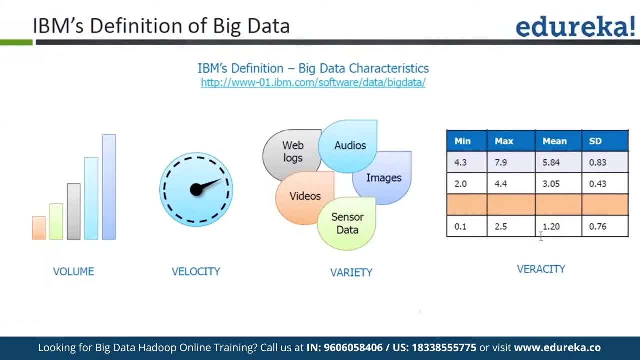 solution. You just cannot go and propose Hadoop to everybody, no matter what problem they have. Somebody says: you know, my email is not going to my manager. You say you cannot do that, right, All right guys. So the point is: how do you know if a business use case? 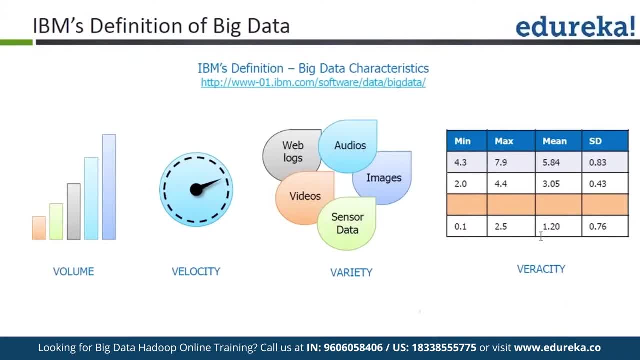 is a Hadoop use case or not. So IBM says there are four different ways of categorizing or tagging your problems as big data, problem or not. right, If you can tag these problems that your clients say into one of the four vertices, then probably these problems are. 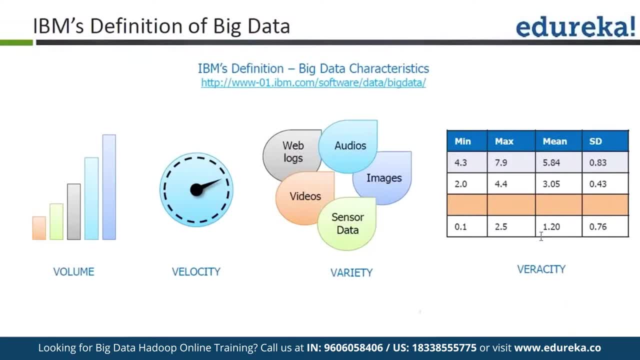 big data problems. The first one is volume. If the client is saying that my data volume is so much and my data is growing so proportionately that I think traditional systems cannot handle that amount of data. If the client says that my data is growing humongously and in a couple 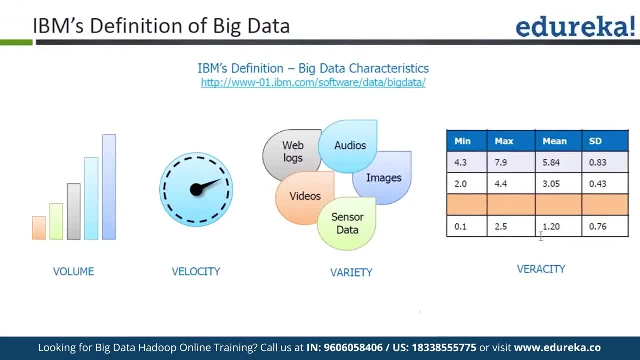 of months. I cannot even imagine where I can keep the data. then Hadoop is the solution for you. So if the data, if the problem is associated with volume, then yes, Hadoop is your solution. Second is velocity. Velocity says: 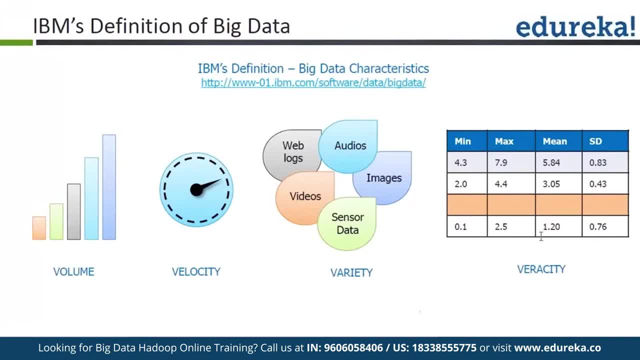 if the rate in which the data has been ingested into your system is so huge that your small system cannot handle that volume, that velocity of data, then Hadoop is great. If you open, if you write a web service, how much events the web service can take for a second guys? 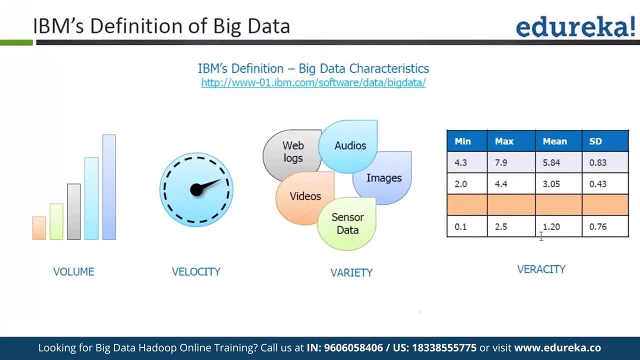 not more than a hundred, right, So it cannot handle more than a hundred requests coming, and there is a sensor which is keeping on sending you data. So nowadays people are talking about IOTs, no internet of things. They're talking about sensors into everything and 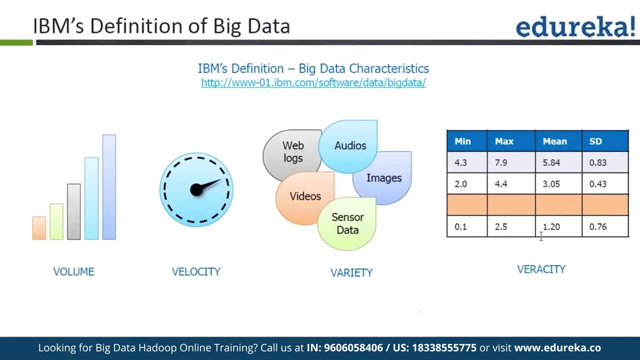 now they're putting sensors into everything. and now they're putting sensors into everything And they have been, you know, pushed down every second. If somebody is sending you millions of events per second, do you think there is any traditional system that can handle that? 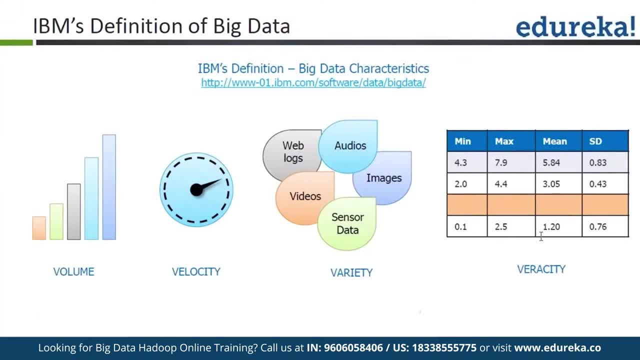 amount of data coming in. No. So if the velocity is a problem, if the data that has been retrieved is so huge that it cannot be processed or cannot be handled by traditional technologies, then Hadoop is definitely for you. Variety, you know, if you want to make a decision and 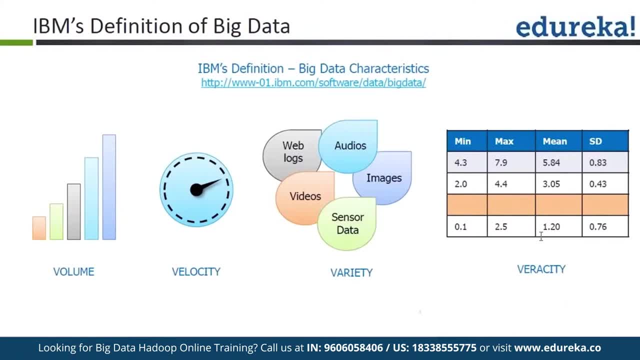 you know that the decision will be based out of a lot of data- and that's something that you can do- And the source of data is varied, and the source and the data itself is also varied. Like you have audio data, video data, log data, text data, CSV data, TSV data, you 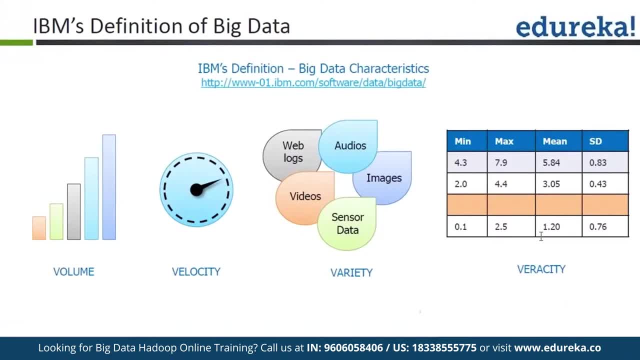 have different kinds of data. If your data is varied and you need to process them together, you know that's the end of the story. You know you have to process them together. Then you need to have a system which can handle, process and analyze this variety of data together. 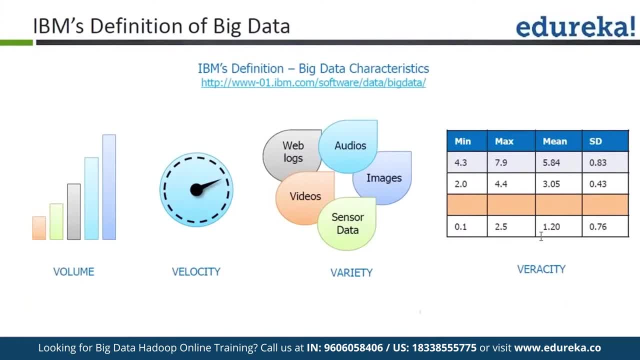 So if variety is a problem, then big data Hadoop is a solution. And then veracity. Veracity says: if the data that is coming for I'm sure about if the data is correct or not, So you cannot save the data. the veracity says: if the data that you are pushing in the data 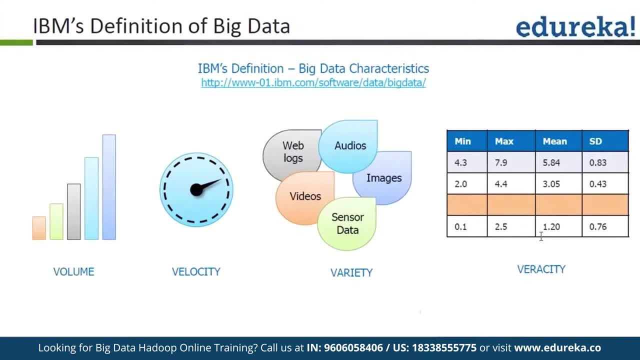 might not be always correct, because you're also talking about data coming from all those external sources. You're not sure about the structure of data. You're not sure if the data is correct all the time. So veracity says: trust the system If you are not sure. 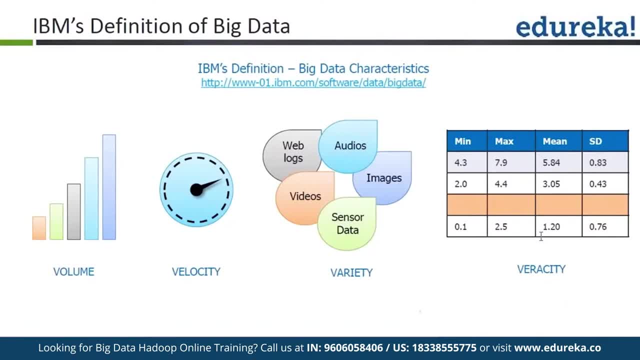 about the kind of data you have. you can still load the data into the data And, if you know, into your H2P system. So veracity says so net about what veracity is in today's world. guys, normally if you talk about 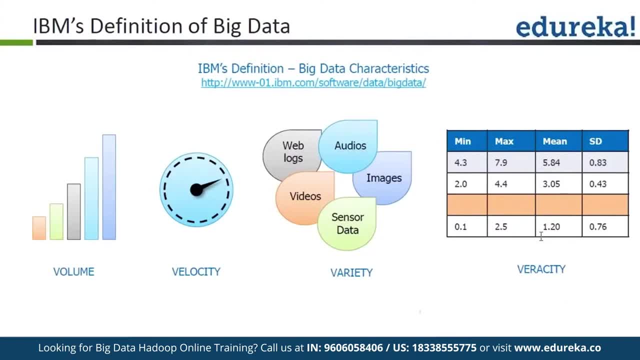 a transactional database, any database you talk about. every data have a shelf life right. Every data have a lifespan. Normally, every year, older data will be archived into a tape, right? You're going to archive the data into the tape and lock the data away? 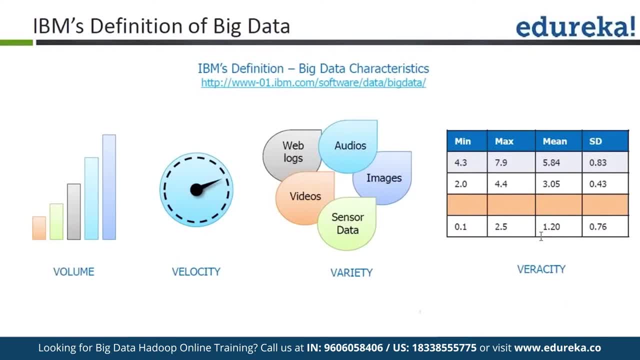 But in today's world you cannot just lock away your data, because data is the most important thing for you. Data is like gold dust. You cannot throw away the data. So Hadoop veracity point says you trust Hadoop with the data. 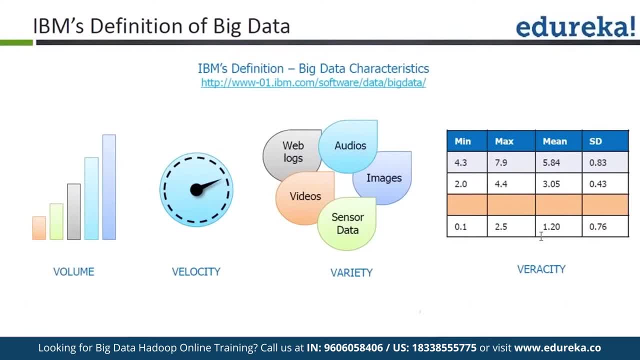 Hadoop says Hadoop is built out of commodity hardware. So we're going to talk about commodity hardware later on. Hadoop is normally based out of commodity. So the net, net important part is setting up and maintaining Hadoop cluster is very, very economical. 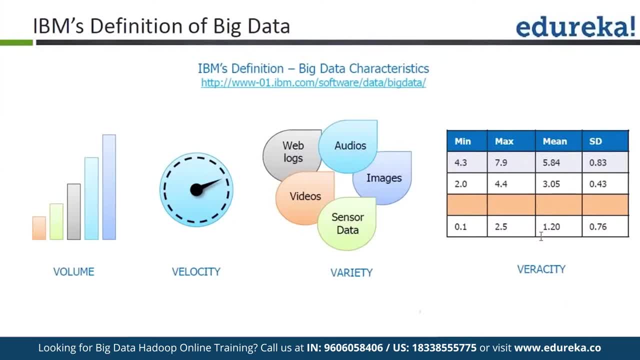 The money you spend on setting up and maintaining Hadoop cluster is quite comparable to maintaining and managing your tapes. So Hadoop says: do not throw away your data, Do not lock away your data. Instead, if you think that you want to archive the data, 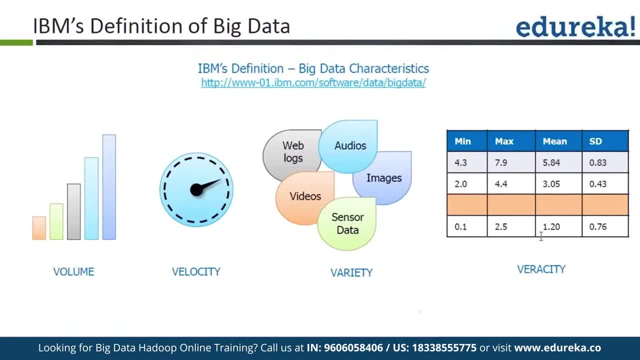 push the data into Hadoop system and you run analytics on the system so that the data is not wasted. If you have 10 years worth of credit card history of a person, you can create models and see and create a front detection model. maybe so important thing, veracity says. 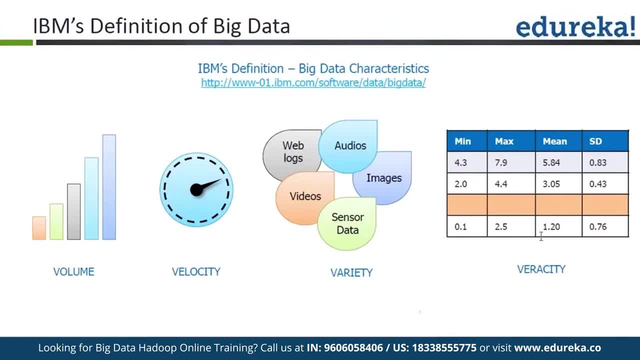 do not throw away the data at any point of time. Do not lock it with the data. Use the data for analytics purposes. You use the data and put the data into a system, into a Hadoop based system, So that later on you can do analytics. 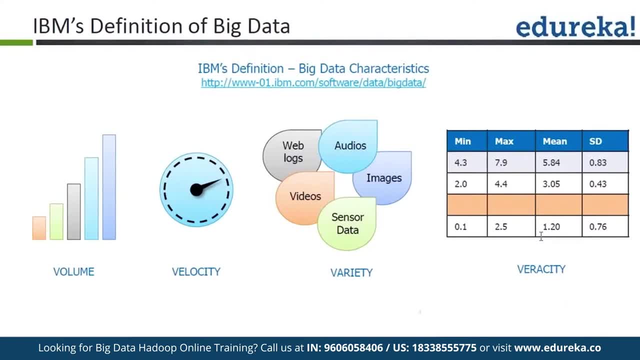 If you're not loud, if you're not, you know thinking about analytics. at this point of time, use Hadoop only for storage, but tomorrow you can go ahead and run analytics on that. So veracity talks about the veracity of Hadoop. 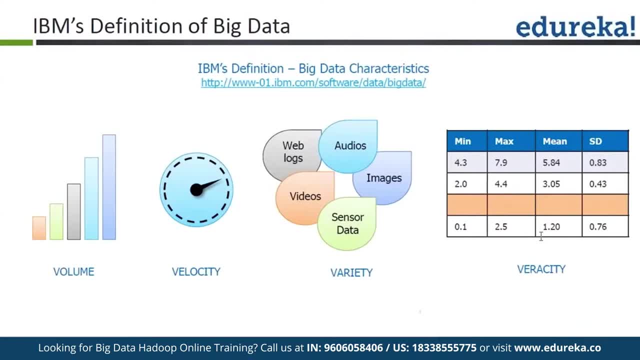 So veracity talks about the veracity of Hadoop. So veracity talks about the veracity of Hadoop. It talks about the value of the data, It talks about the trust of the data and it talks about the ease of which you can load the data.